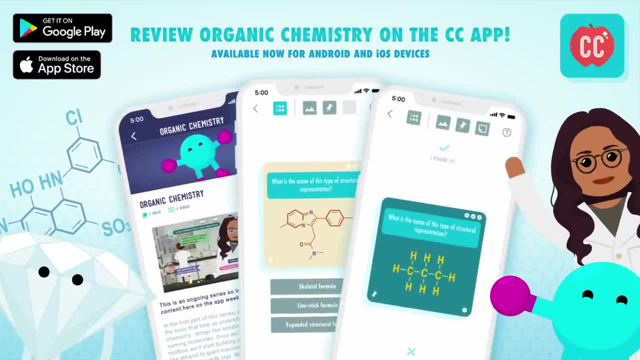 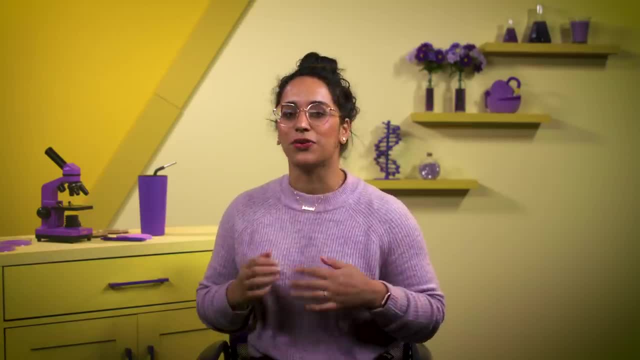 You can review content from Crash Course Organic Chemistry with the Crash Course app, available now for Android and iOS devices. Hi, I'm Deboki Chakravarty and welcome back to Crash Course Organic Chemistry. Movies and TV shows are full of instant science. 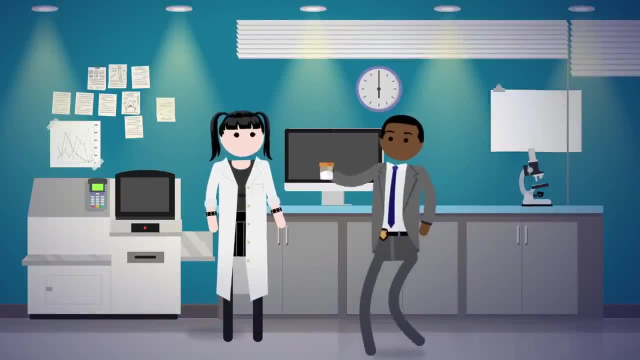 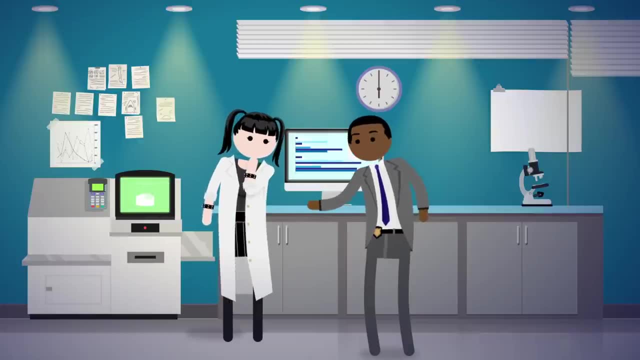 A TV cop brings back a mysterious white powder from some crime scene and lab techs run it through a machine. Seconds later, the substance is identified with a science-y looking graph and the tech says something like I thought. so it's powdered sugar. 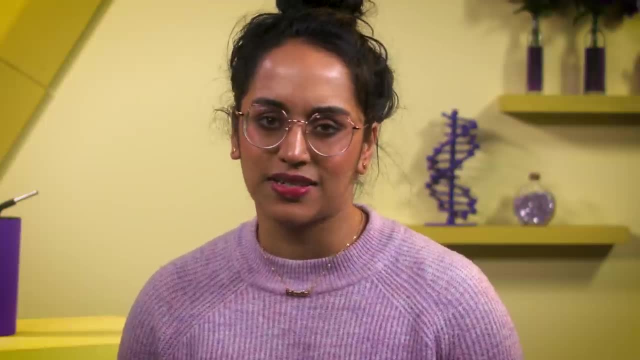 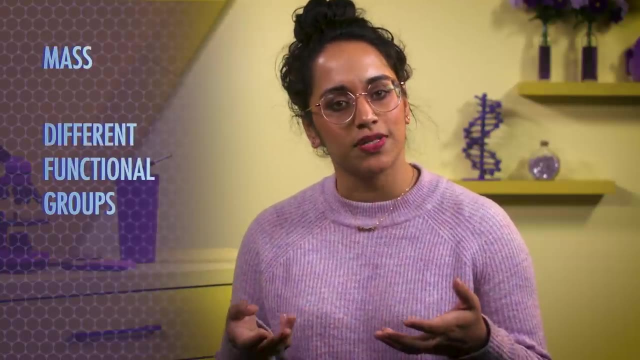 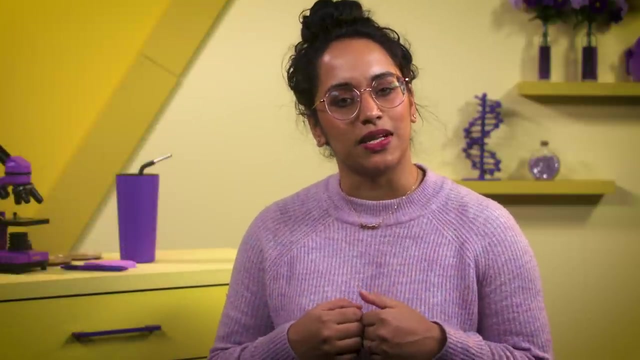 Reality is not so clean or easy or fast. TV has it right on one level. We can use instruments to learn things about molecules, like their mass, different functional groups or what geometric isomer they are. But it's not so easy to know what you're looking at and it usually takes a couple instruments to get a more conclusive answer. 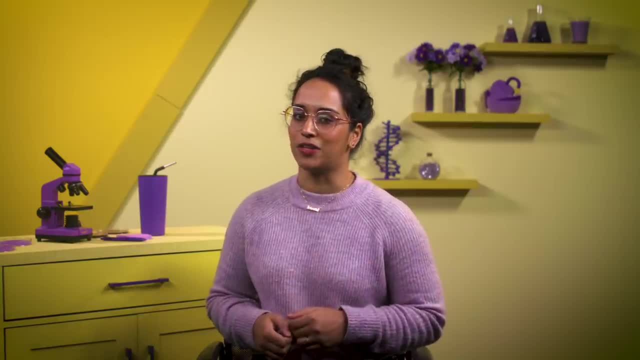 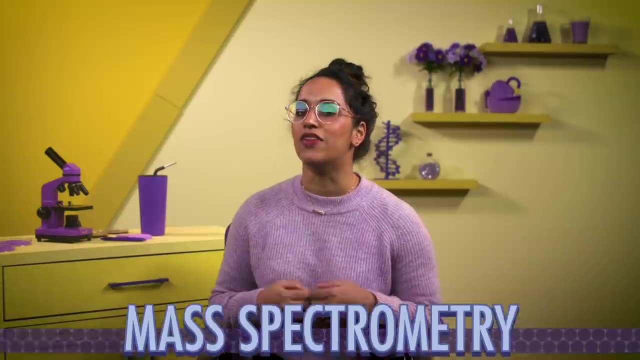 Today we'll look at two important tools that we can use to examine molecular compounds: infrared spectroscopy and mass spectrometry. And to make it fun, we'll do it through the lens of a forensic investigation. Let's set the scene. 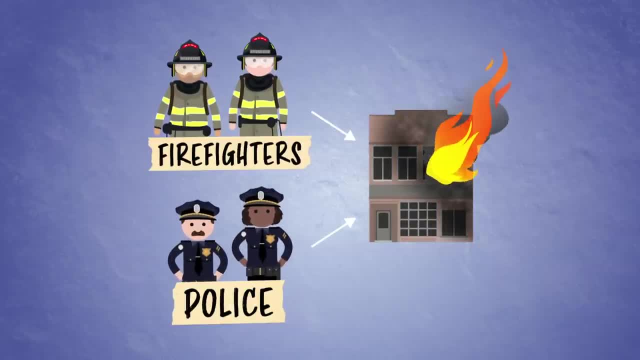 Firefighters and police are called to an explosion in a building. After the fire is contained, evidence is collected. Among lots of samples, investigators find what looks like chemistry lab equipment and some white powder in part of the building not affected by the explosion or the firefighting chemicals. 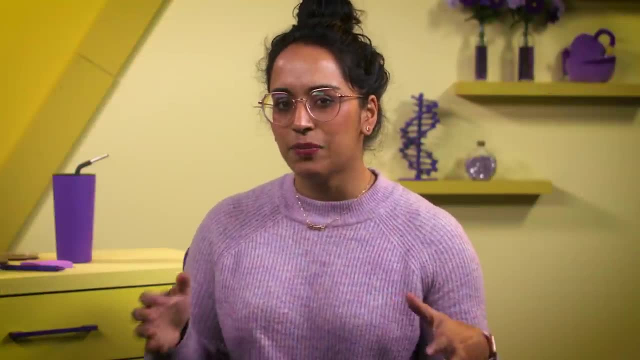 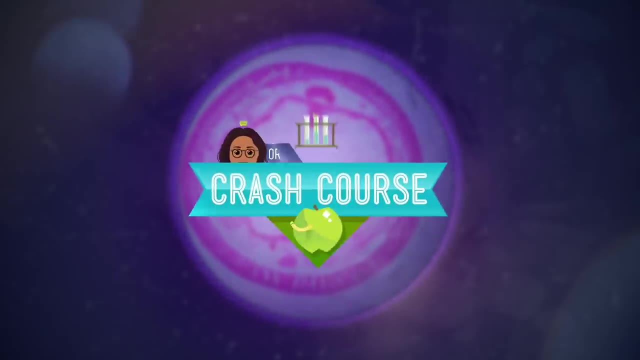 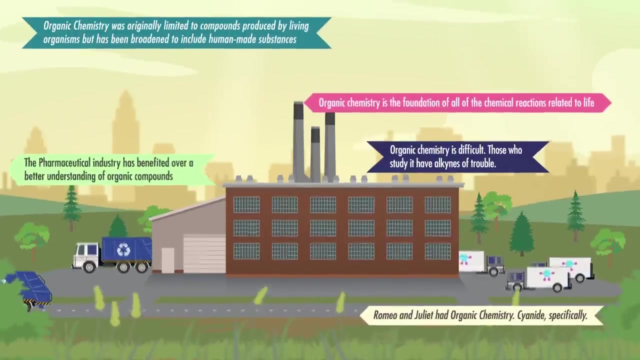 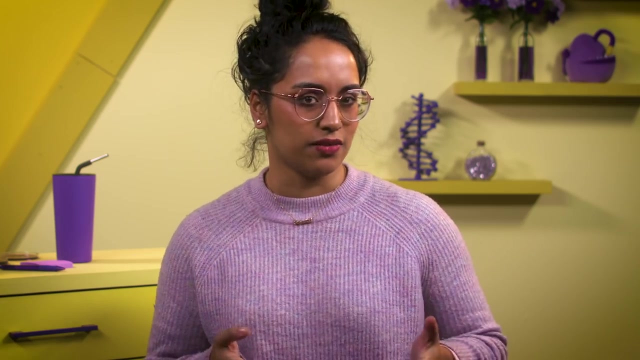 Now let's step into the shoes of the crime scene techs. A sample of white powder has been delivered to us And it's our job to identify it. Time for molecular analysis. Before we get too deep into our mystery, we need to set something straight. 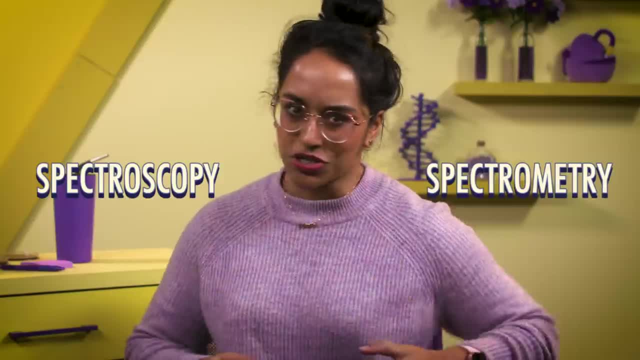 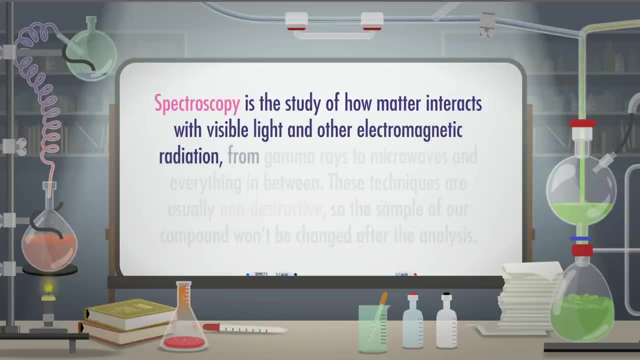 Spectroscopy and spectrometry are not interchangeable words. Spectroscopy is the study of how matter interacts with visible light and other electromagnetic radiation, from gamma rays to microwaves and everything in between. These techniques are usually non-destructive, so the sample of our compound won't be changed after the analysis. 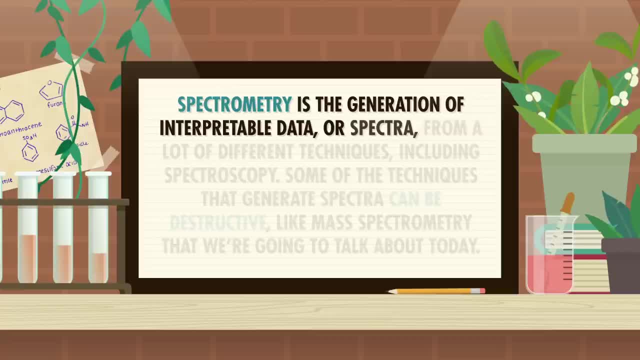 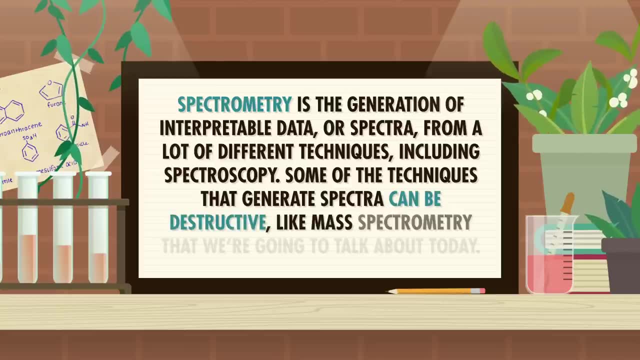 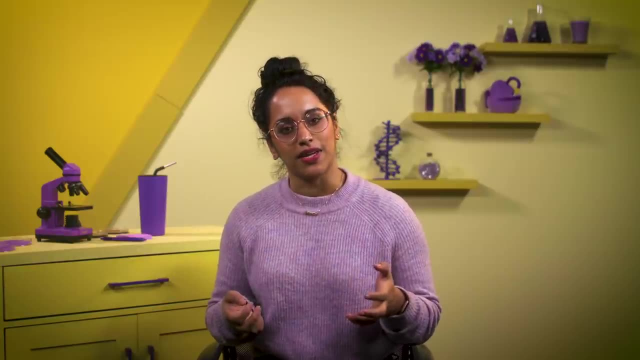 Spectrometry is the generation of interpretable data or spectra from a lot of different techniques, including spectroscopy. Some of the techniques that generate spectra can be destructive, like mass spectrometry that we're going to talk about today. Basically, the main difference is that spectroscopy is just observing how electromagnetic radiation interacts with molecules. 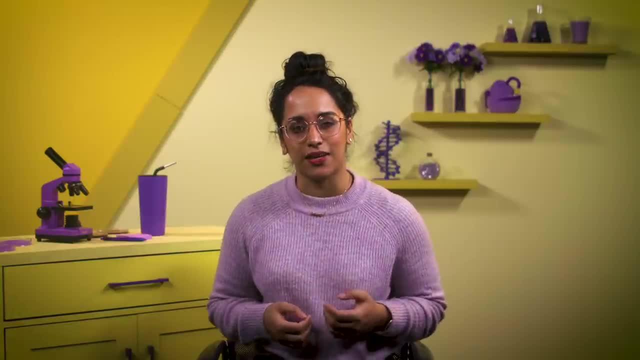 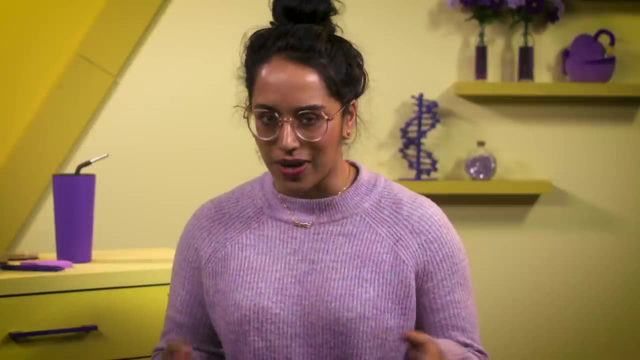 while spectrometry provides data that we can use to interpret the structure. Both of them can be used for individual substances or mixtures, But mixtures are way more complicated, so we'll stick to one substance at a time for now. Okay, now that we've cleared that up, let's dive into the techniques. 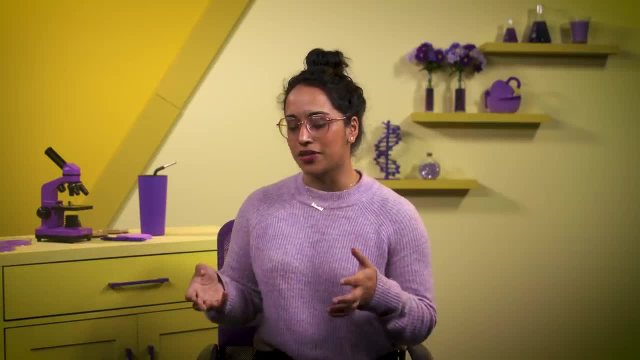 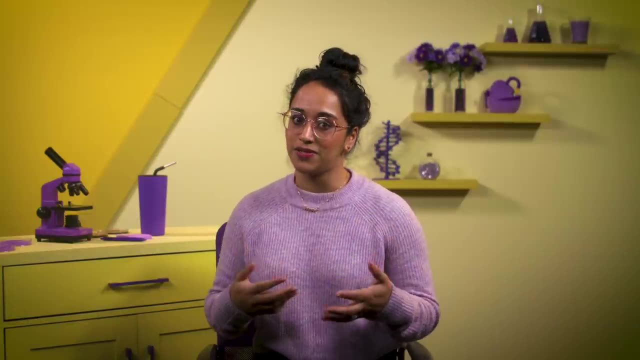 Using a very small amount of sample. mass spectrometry, or mass spec for short, gives us information about a molecule's molecular mass, which is the added-up weights of all its atoms Inside a mass spectrometer. there aren't any errors. 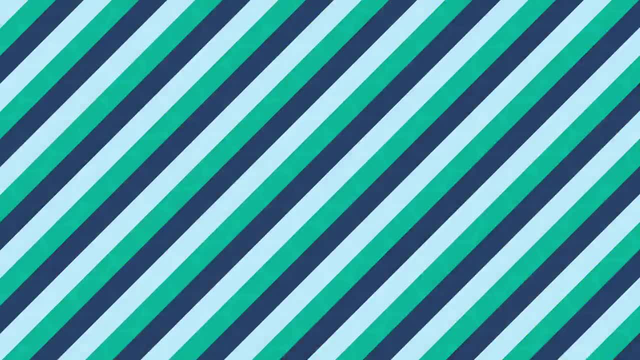 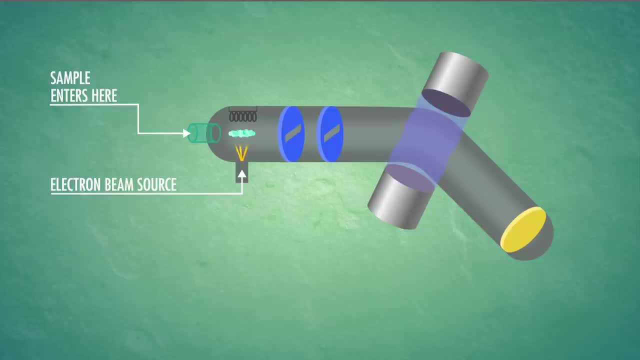 There are particles whizzing around, so it's a vacuum like outer space. A sample molecule goes into a chamber and the ion source generates a stream of electrons with a high-temperature electrical current. In the ion source, a metal gets zapped, electrons get liberated and that electron stream hits the sample molecule. 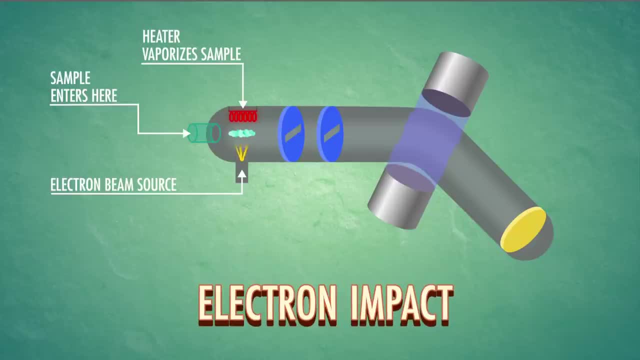 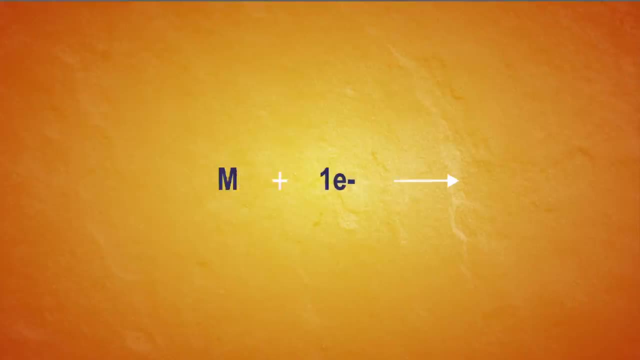 This technique is called electron impact. It's a destructive approach, but also one of the most common in mass spec. When this stream of focused electrons strikes a molecule, an electron splits off from the molecule and forms a radical cation. It leaves behind an unpaired electron, a radical. 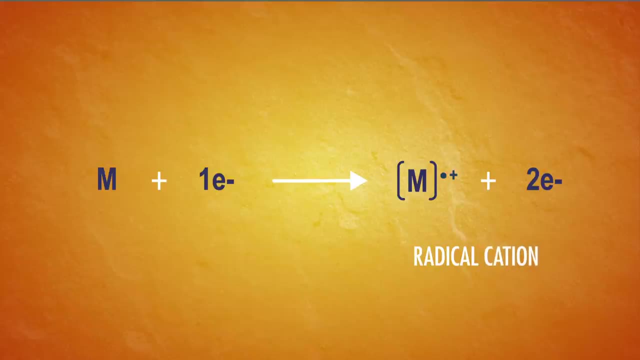 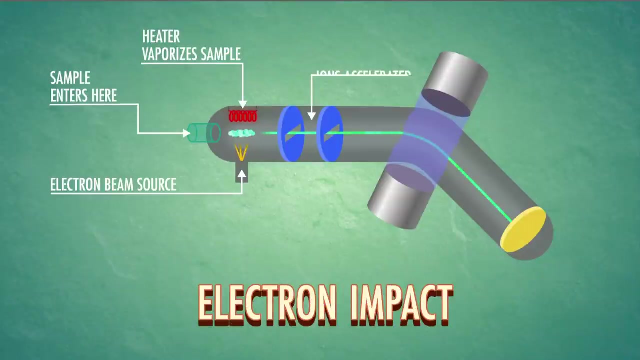 And it's a cation with a positive charge. because a neutral molecule loses an electron. This radical cation is called the molecular ion. In an ideal situation it flies down the tube of the mass spectrometer to the detector. as-is. However, electron impact is sort of like a bullet hitting a glass bottle, so sometimes the sample molecule is broken apart into other ion fragments. 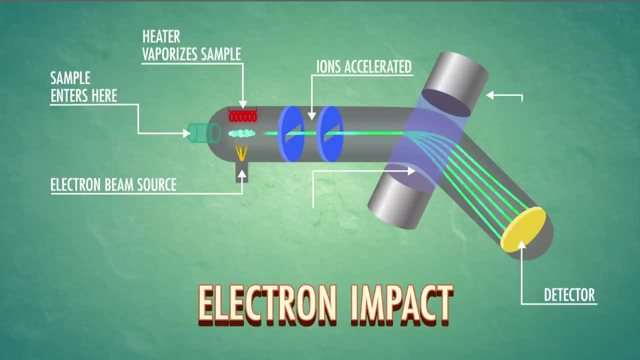 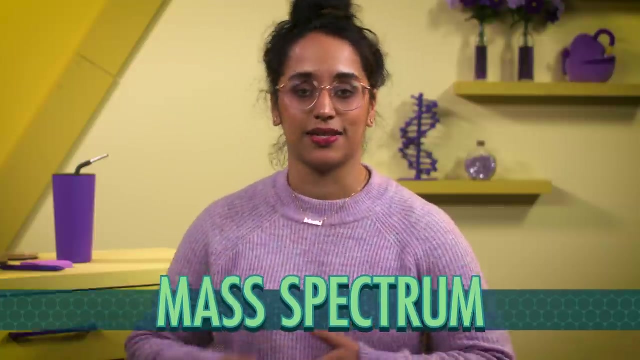 Any molecular ions and ion fragments are sent down a tube where a variable magnetic field sorts them by mass. This way, only particles of a specific mass can hit the detector at one time. Then a mass spectrum is produced, with mass on the x-axis and the relative number of ions on the y-axis. 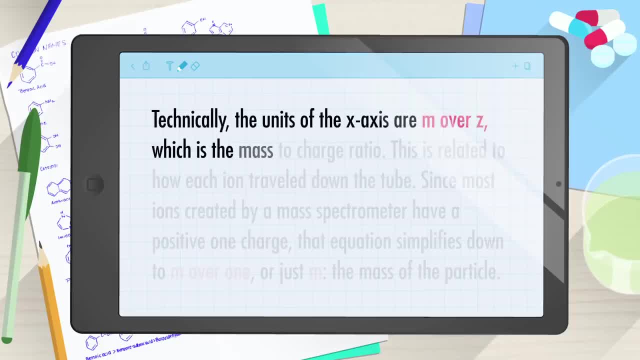 Technically, the units of the x-axis are m over z, which is the mass-to-charge ratio. This is related to how each ion traveled down the tube, Since most ions created by a mass spectrometer have a positive one charge. the equation simplifies down to m over one, or just m, the mass of the particle. 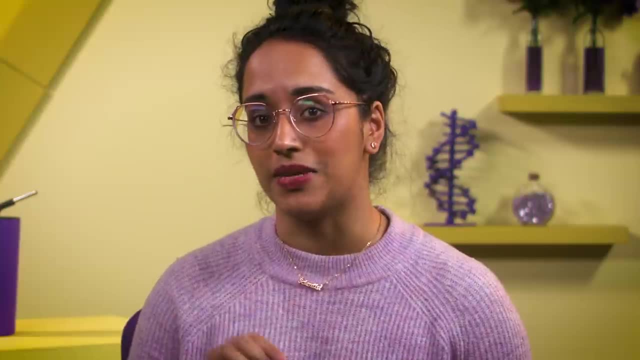 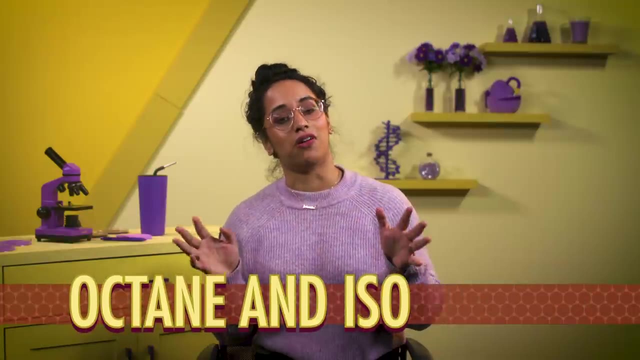 Now the molecular fragments hitting the detector form a fragmentation pattern that's unique to the molecule. For example, let's look at mass spectra for octane and iso-octane, or 2,2,4-trimethylpentane, if you want to be IUPAC official. 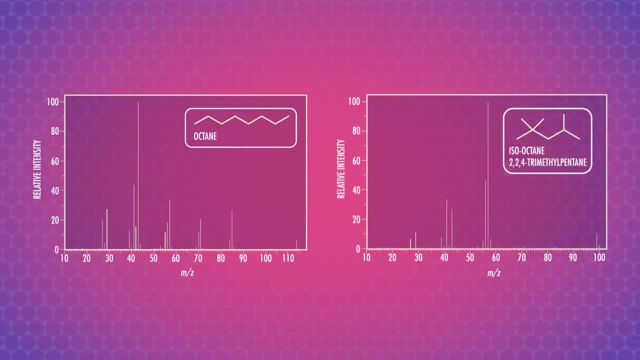 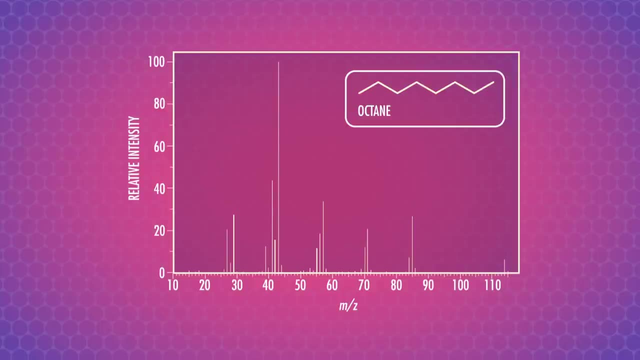 Both molecules have the same molecular formula and therefore the same molecular mass of 114 mass units. But mass spec can tell the two apart. Starting with octane, we notice that the rightmost part of the mass spectra is the mass spectra. 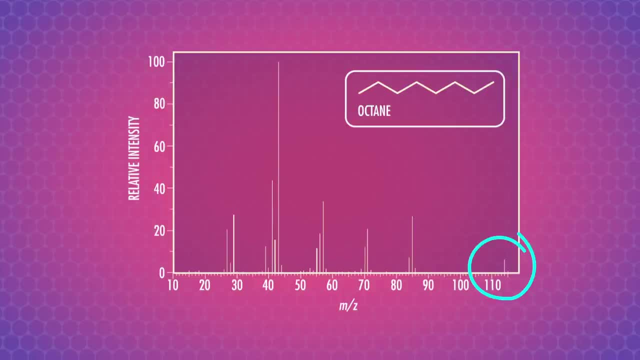 This peak on the mass spectrum shows up at 114 m over z. Knowing the molecular mass of octane, 114 mass units, we know that peak is the molecular ion. If we subtract the next highest peak, so 114 minus 85,, the difference is 29 mass units. 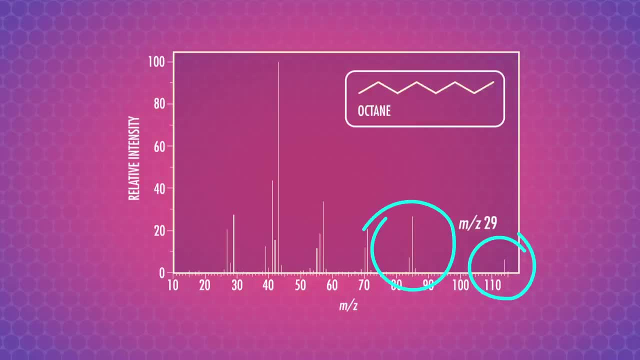 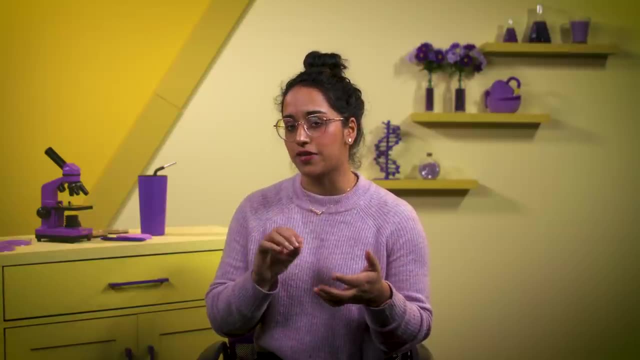 This means that the octane molecules split into two chunks here: one of 85 mass units and one of 29 mass units. It's often easier to identify the smaller fragment that split off than the big one that got left behind and made the difference. 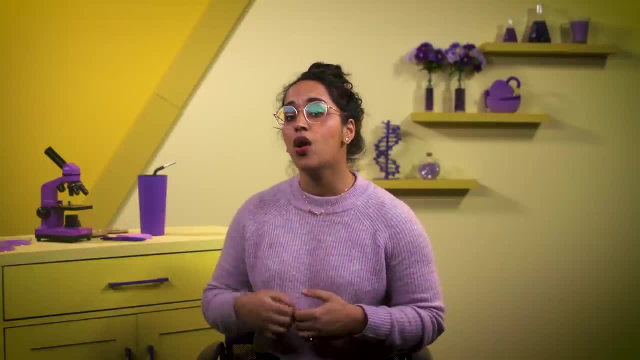 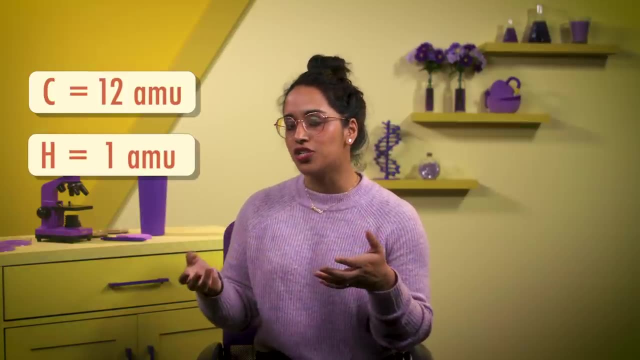 To figure out what the 29 mass unit piece is. we know that one carbon has a mass of 12, and each hydrogen has a mass of 1.. Then we can add more carbons and hydrogens until we get to 29.. 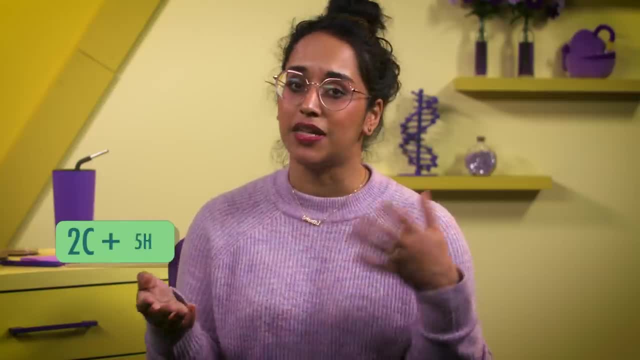 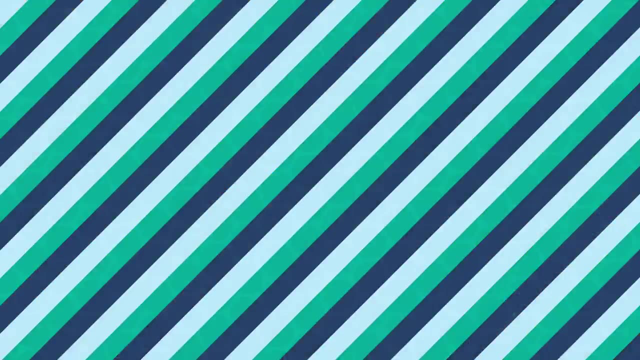 In this case, 2 carbons is 24 mass units plus 5 hydrogens is 29 mass units. This gets us to CH3CH2, an ethyl group fragment. This means that the 85 m over z peak is whatever's left of the octane when an ethyl group splits off. 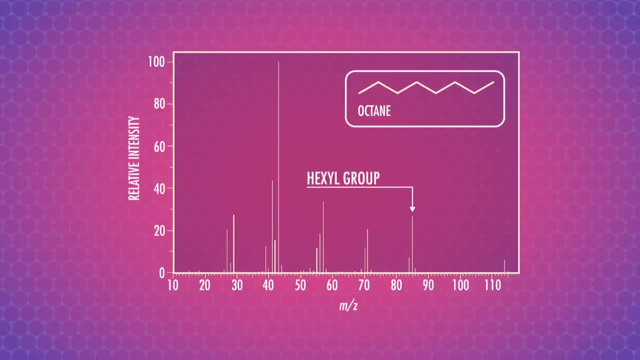 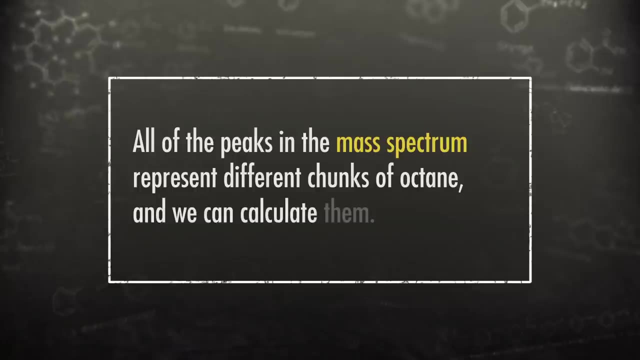 So it's a hexyl group. There's always a bit of trial and error, but that's what we chemists do best. All of the peaks in the mass spectrum represent different chunks of octane, and we can calculate them, But here's one peak that's very important to organic chemists – the base peak. 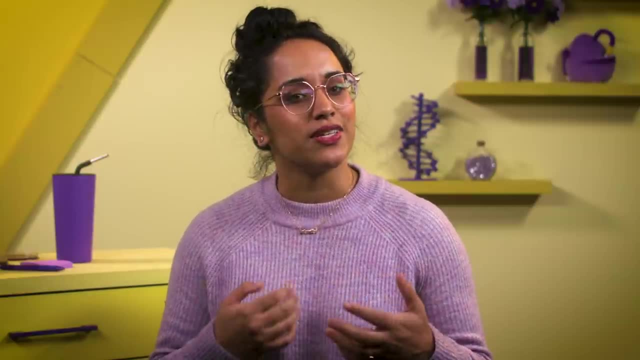 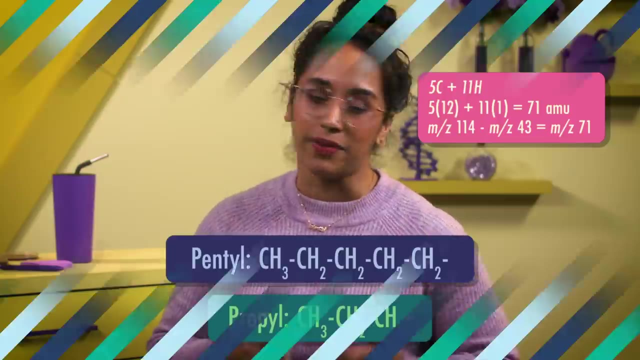 This is the tallest peak, at 43 m over z. If we do the same math, we know that corresponds to a pentel fragment splitting off and a propyl group left over, which is what's causing the peak. The propyl group having the tallest peak means that it has the highest relative intensity. 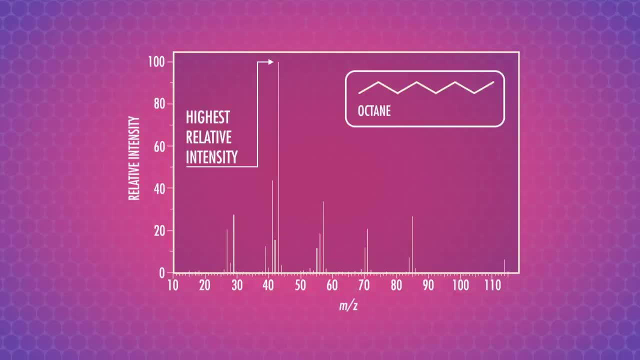 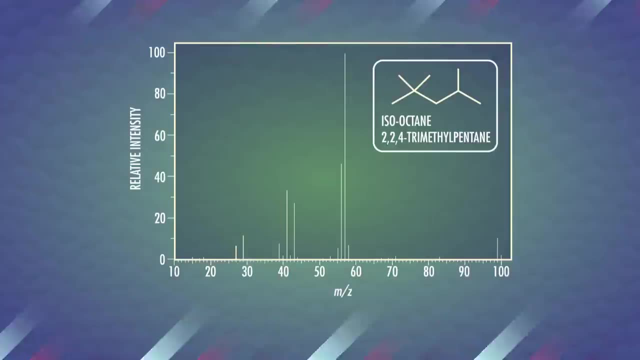 and it's the most stable ion that forms in the fragmentation. Sometimes the most stable fragment can tell us a lot about the structure of a compound. Switching over to the spectrum for iso-octane we can see the pattern is very different. 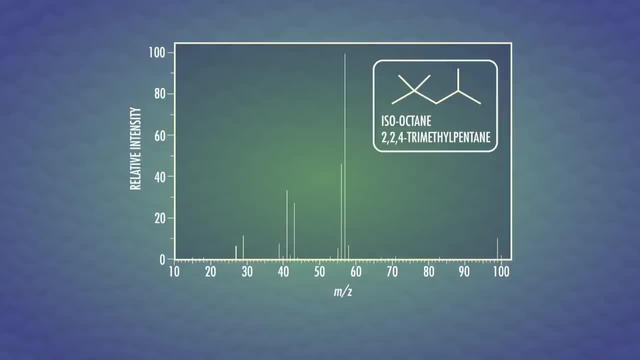 We know its molecular mass is also 114 mass units, so we can see that the molecular ion isn't there. The highest recorded mass is that small blip at 99 m over z, and 114 minus 99 is 15 mass units. 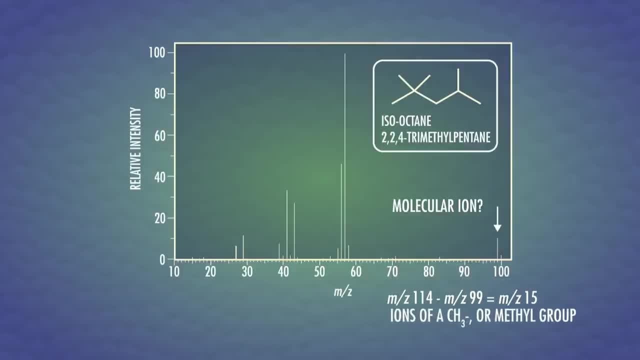 Which corresponds to the loss of a CH3, or methyl group. The base peak is 57 m over z and using the same math we can figure out that this is a 4-carbon group with 9 hydrogens. The branching of iso-octane leads to a very different base peak from octane. 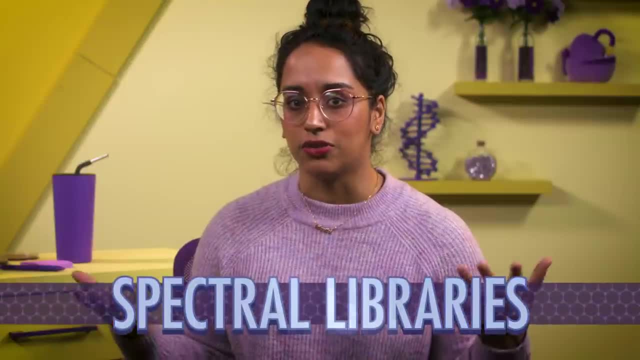 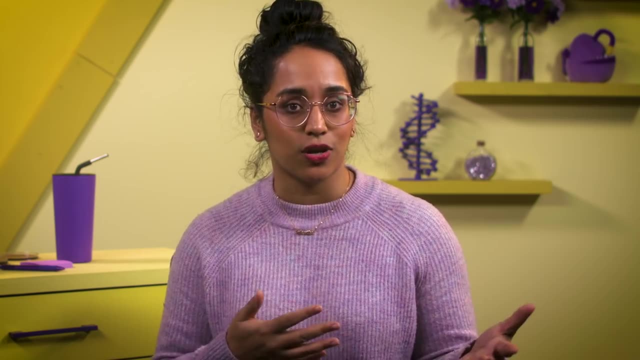 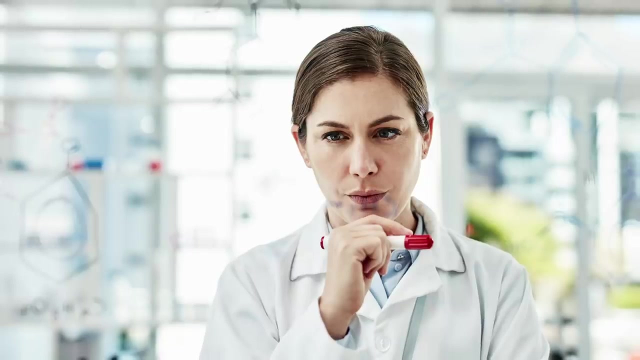 Over the years we've developed databases called spectral libraries, which contain known spectra of different molecules. Most operating programs can search through thousands of libraries to give us the most likely matches. But even with the help of computer programs, we still need to use our human brains to think critically and check whether the fragments make sense for our experiment. 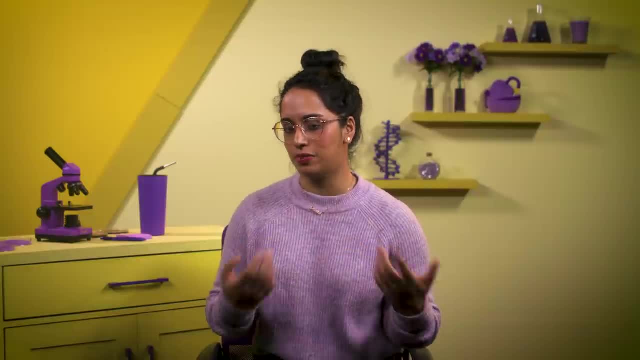 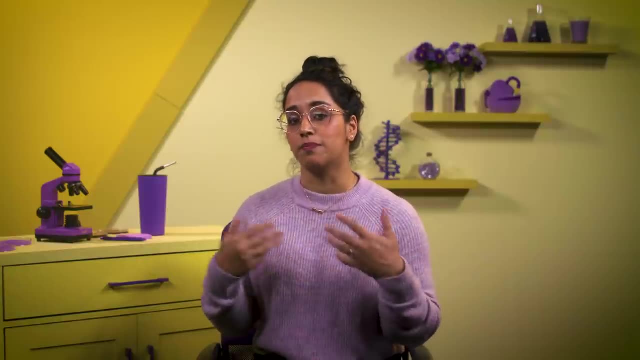 Now that we have one tool, let's go back to the mystery white powder from that exploding building. If we run a mass spec experiment, in about 30 minutes we'll get a spectrum. Then we can ask the program to run a comparison with a library of spectra to help us identify our molecule. 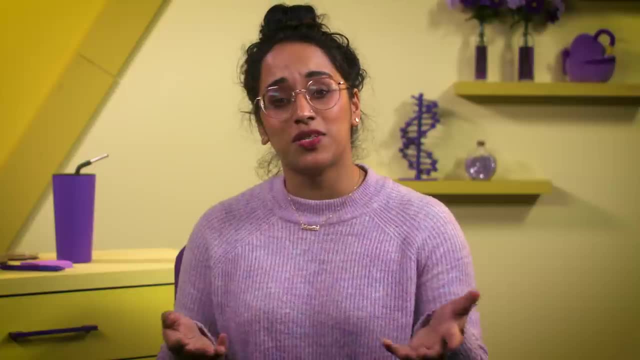 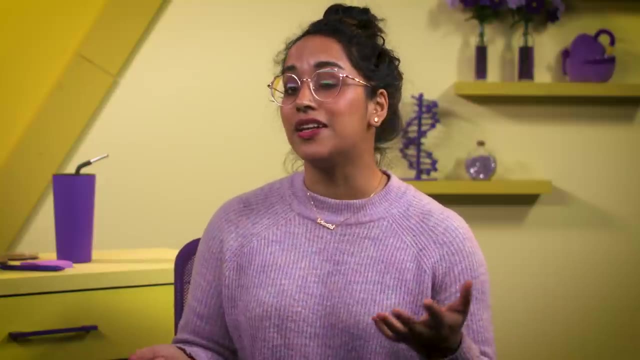 But the library spits out around 605 matches. There are 605 different spectra that could be the spectra for our mystery powder. To narrow this down and get a better sense of the chemical formula it might have, we can use a slightly modified version of this tool. 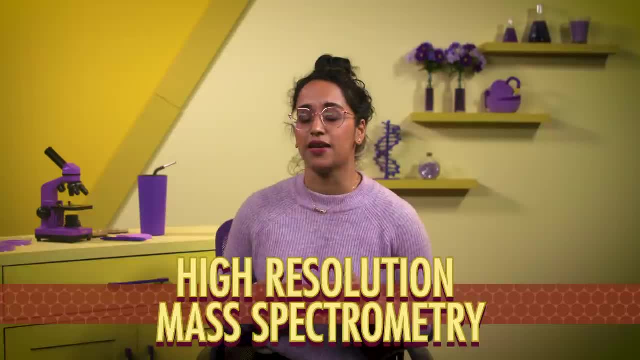 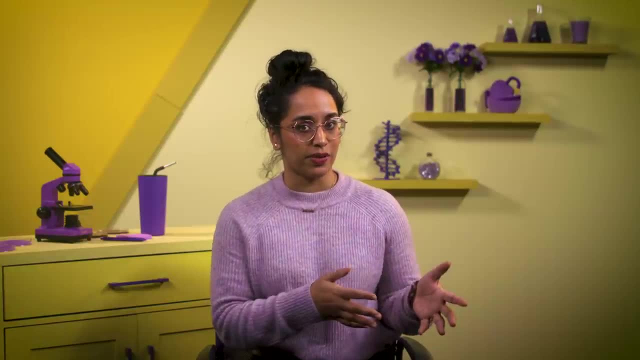 High-resolution mass spectrometry is a more sensitive technique with a more focused electron beam that lets us determine the exact mass, which is the molecular mass, to more decimal places and therefore more certainty. We can use the exact mass along with the molecular mass databases to identify the molecular formula. 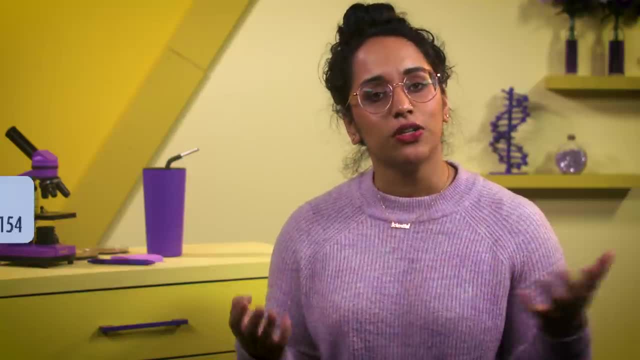 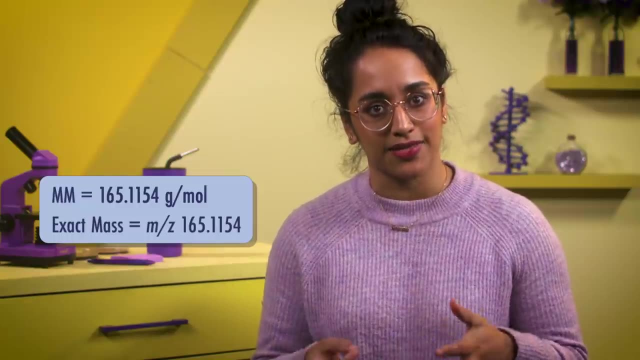 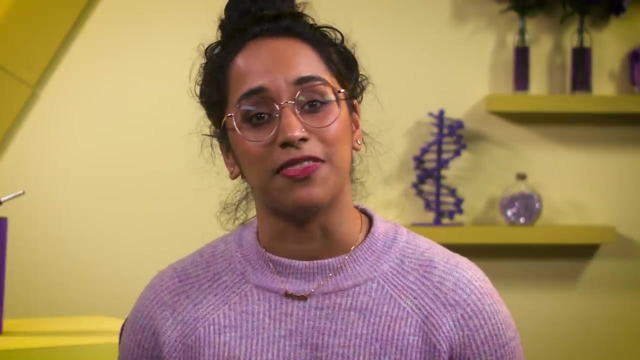 After doing this high-res mass spec on our substance, we learned that the molecular mass is 165.1154 grams per mole, And the published tables of exact mass and molecular formula lead us to C10H15NO. The top match for this fragmentation pattern and formula in the mass spec library is 2-methylamino-1-phenylpropan-1-ol. 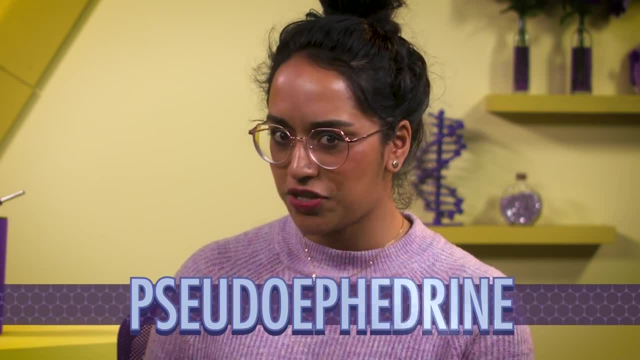 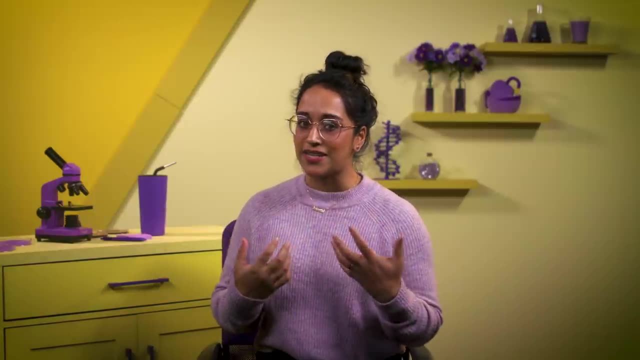 And the program gave us the common name too – pseudoephedrine. So we're getting closer, But this white powder is coming up. It's coming from a crime scene, And our crime lab training tells us that pseudoephedrine can be used to make methamphetamine. 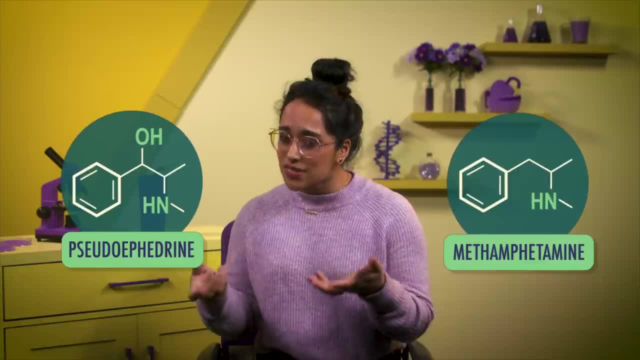 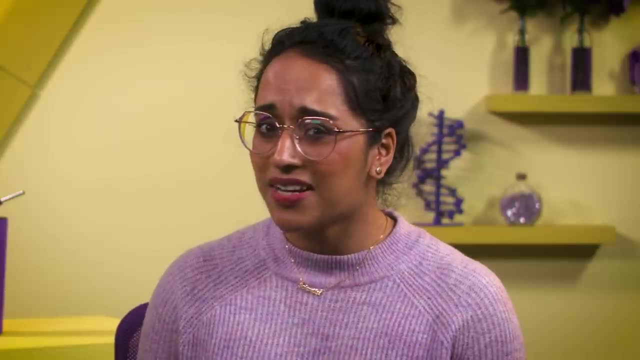 And the molecules are pretty similar, So it's better to have some more data to support our claim. Mass spectrometry can tell us important things, But alone it might not give us information about molecular structure or what functional groups are present. This is where infrared spectroscopy can help. 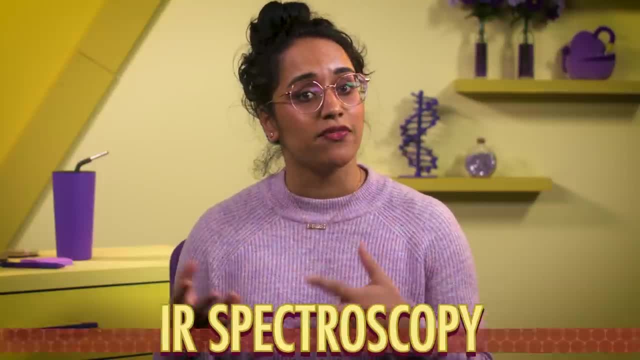 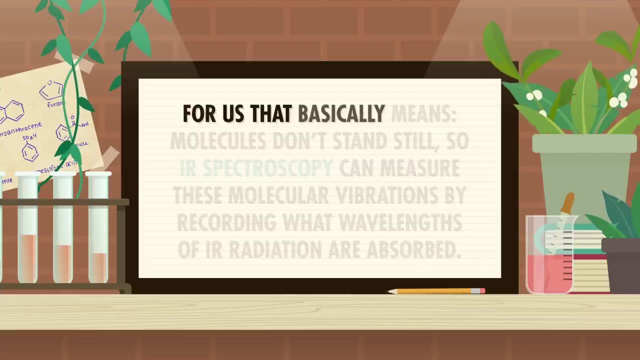 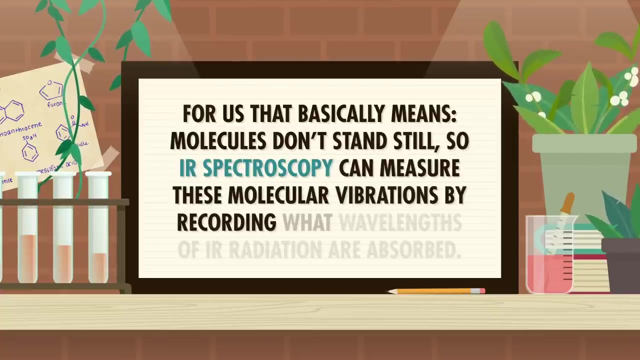 Infrared or IR spectroscopy is the study of how light in the infrared region of the electromagnetic spectrum of the electromagnetic spectrum, interacts with stuff. For us that basically means molecules don't stand still, so IR spectroscopy can measure these molecular vibrations by recording what wavelengths of IR radiation are absorbed. 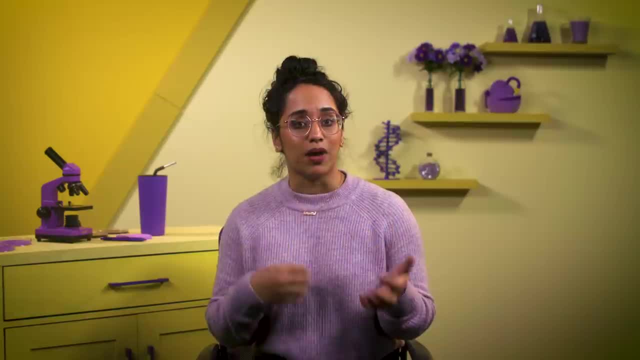 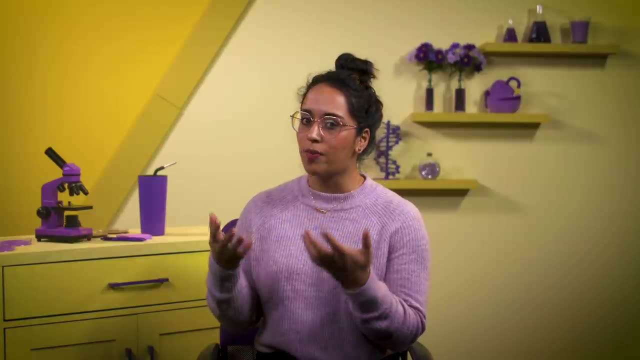 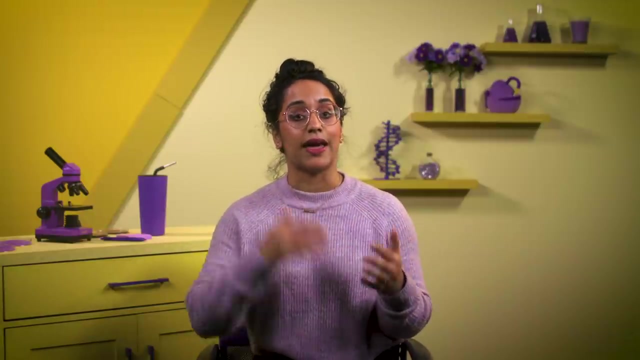 To think about molecular vibrations. we can think of molecular bonds as springs with atoms attached. Stronger springs take more energy to move around, so molecules with stronger bonds need to absorb light with more energy to keep those vibrations going. A triple bond will absorb light at a higher energy than a single bond. 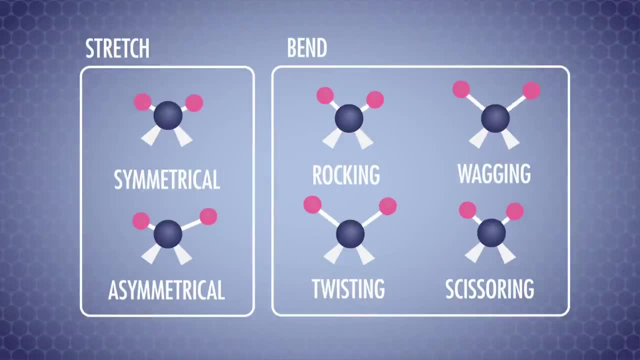 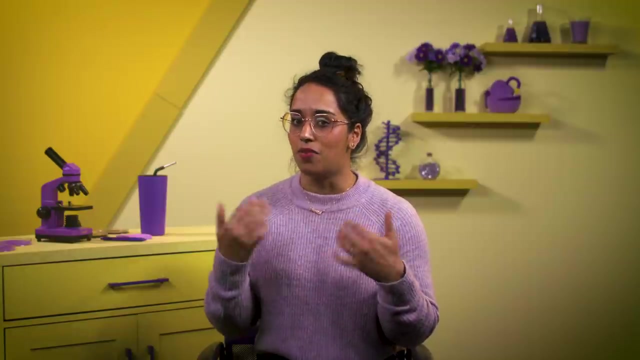 Bonds within molecules can vibrate in different ways, like a stretch, a wag and a bend. All these dancey-sounding motions need different wavelengths of IR radiation. So basically, IR spectroscopy involves blasting a molecule with IR radiation and seeing what gets absorbed as the molecule's bonds vibrate. 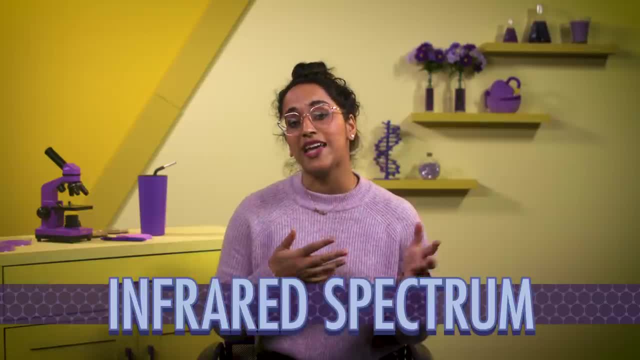 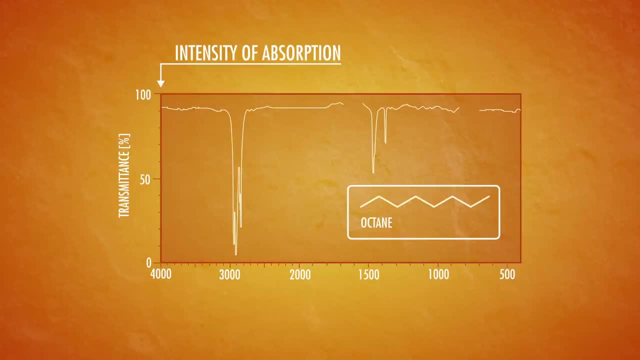 Then an infrared spectrum is produced and we can use it to help figure out what molecule it is. The y-axis is the intensity. The y-axis is the intensity of the absorption, which is related to the kind of molecular motion. Some vibrations are more intense than others. 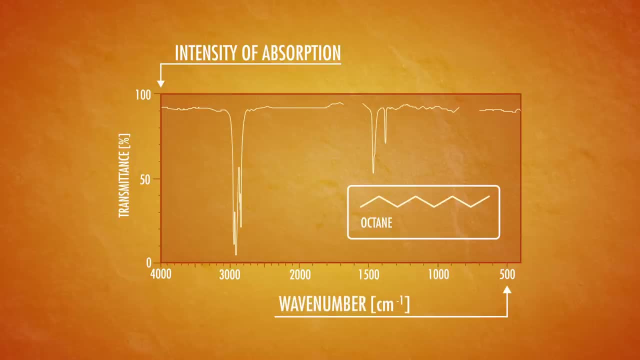 And the x-axis uses wavenumbers as the units. It's a complicated energy term, so for the sake of this already tricky concept, we're just going to say that higher wavenumbers mean higher energy absorption. So let's compare the IR spectra of octane, oct-1-ene and oct-1-i. 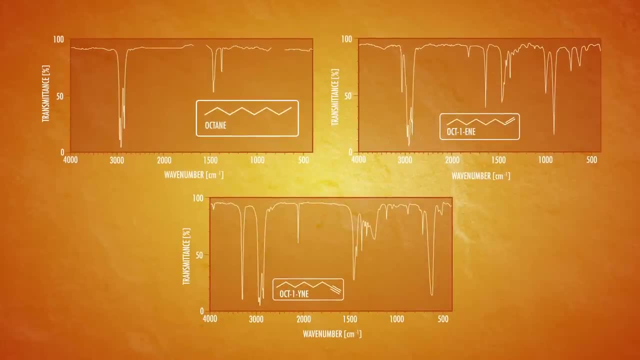 Carbon-hydrogen stretches occur around 3,000 wavenumbers. Looking at the octane spectrum, we see a nicely defined set of peaks around 3,000 wavenumbers. In the oct-1-ene spectrum, the peak slightly to the left of the CH stretches is the hydrogen next to the double bond. 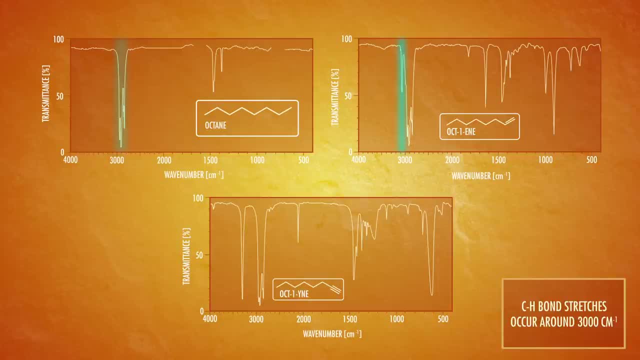 Because the double bond is a stronger bond. its CH stretch has higher wavenumbers. Finally, in the IR spectrum of oct-1-yne that sharp peak is even further to the left and at higher wavenumbers because it marks the CH stretch of the triple bond. 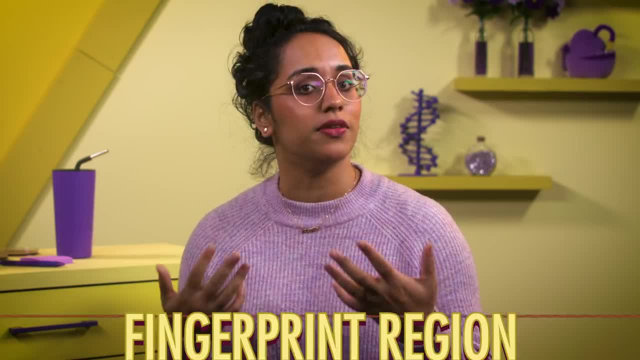 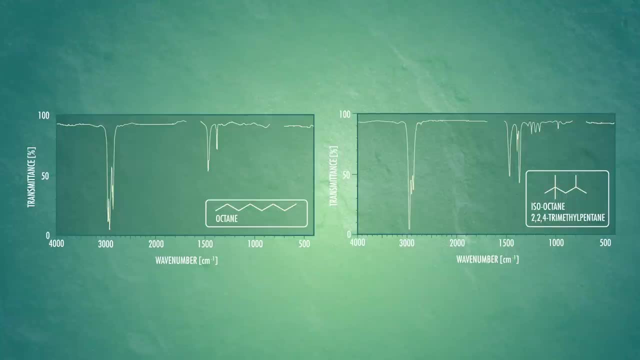 The region of an IR spectrum that's most complex is called the fingerprint region, Kind of like our fingerprints. This region gives us a clue to more complicated molecules. For example, let's compare our old friends octane and iso-octane. Look at the region from 1,400 to 600 wavenumbers. 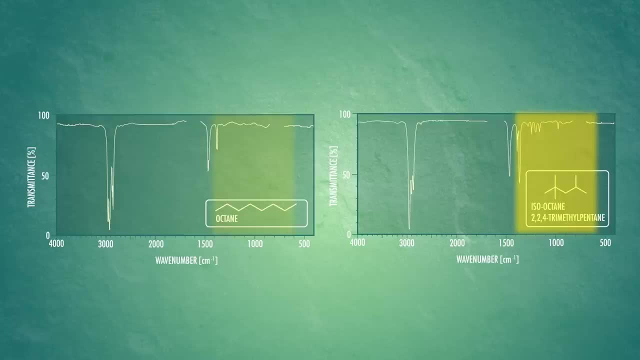 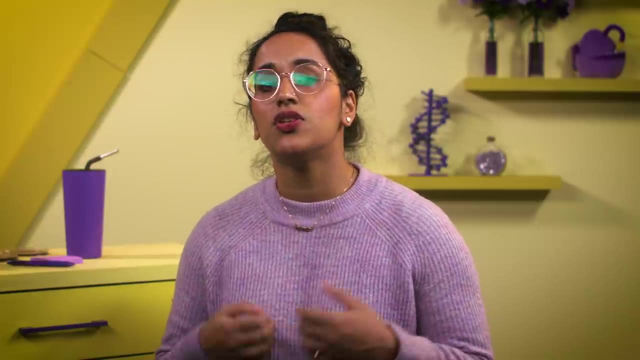 Because iso-octane has more complicated connections between atoms, its fingerprint region is more complicated. But aside from this kind of comparison, it's pretty hard to interpret fingerprint regions. So we usually look for bigger structural clues, around 3,000 to 1,000 wavenumbers, like functional groups. 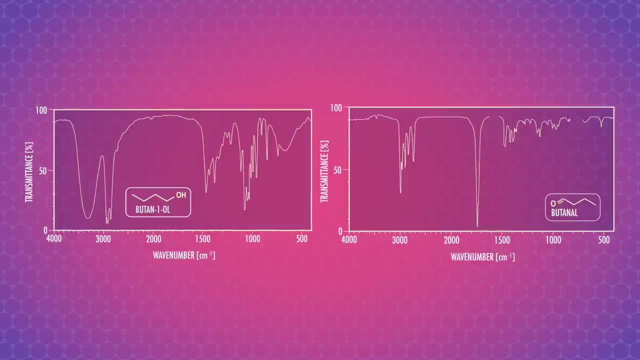 Let's look at IR spectra for the molecules butan-1-ol and butanal. The fingerprint regions are different, but there are other differences that let us quickly identify some functional groups. Looking at butanal, there's a super sharp and strong peak at 1,731 wavenumbers, which indicates the carbonyl group. 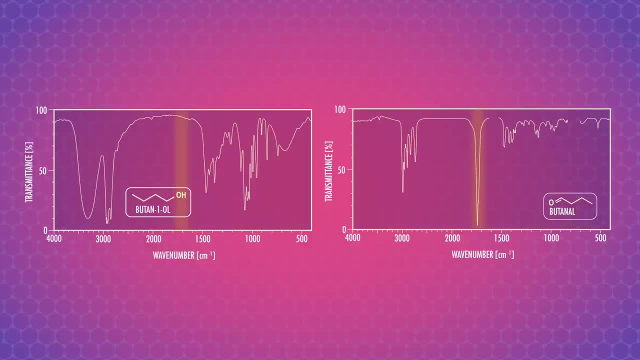 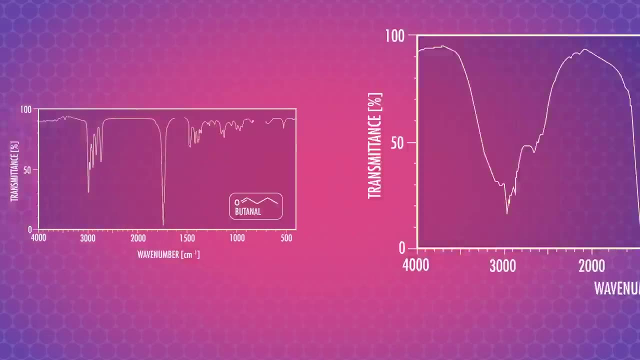 This peak is missing in butan-1-ol because it doesn't have a carbonyl group, But there is a strong broad peak at 3,300 wavenumbers which indicates the alcohol group. To double check this, we can look at butanoic ads.